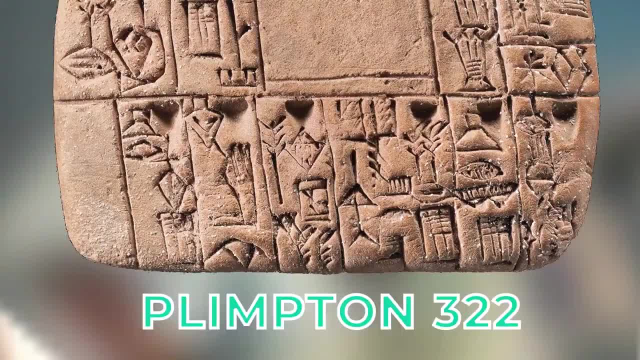 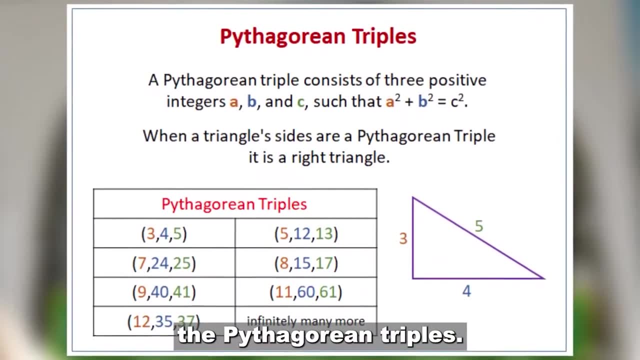 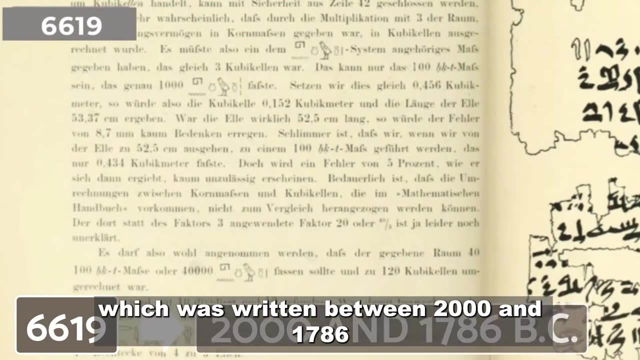 A Mesopotamian tablet, the Plimpton 322,, which was written during the reign of Hammurabi the Great, purportedly contains entries that are related to or resemble the Pythagorean triples. Meanwhile, the Middle Kingdom, Egyptian Berlin, Papyrus 6619,, which was written between 2000 and 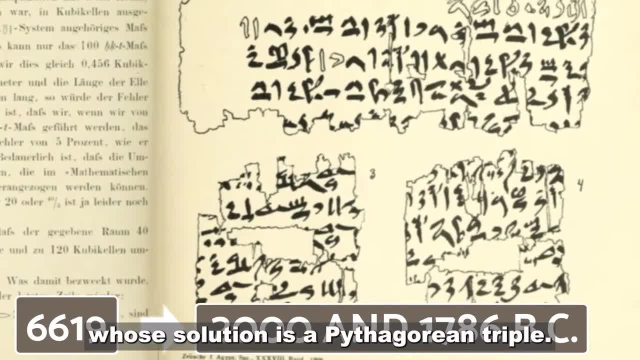 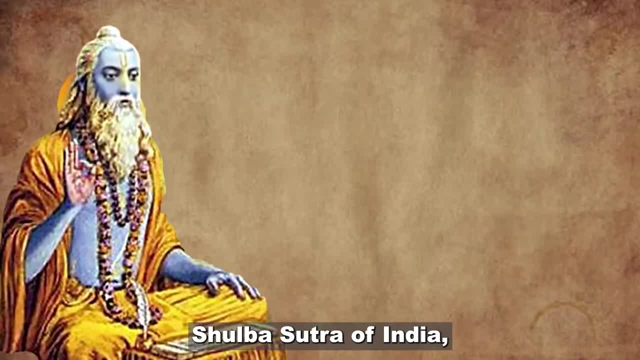 1886 BC is also said to contain a problem whose solution is a Pythagorean triple. However, triangles are not mentioned in it. To add to that, the Baudhyana Shubha Sutra of India, which was said to have been created between the 8th and 15th century BC, also contains entries. 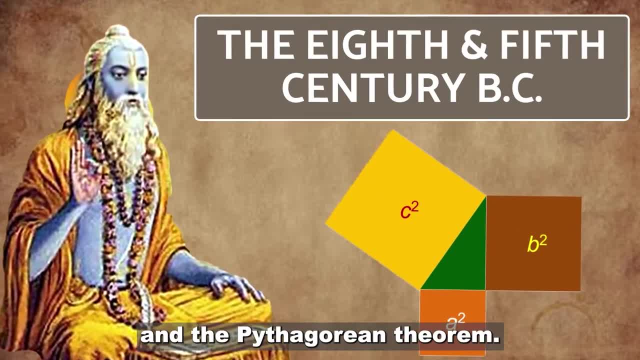 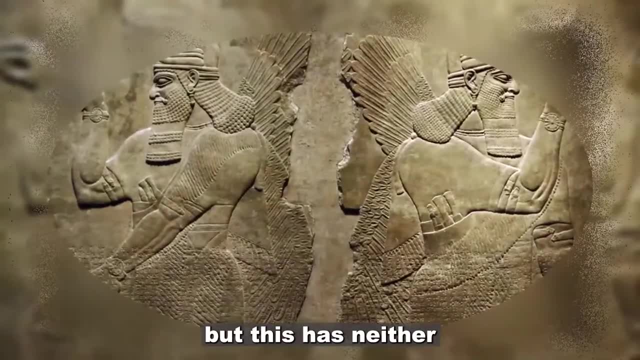 that list out the Pythagorean triples and the Pythagorean theorem. Some historians believe that these texts were based on the mathematics of the ancient Mesopotamian civilization, but this has neither been proven nor disputed. Now, how is the Pythagorean theorem used in real life? 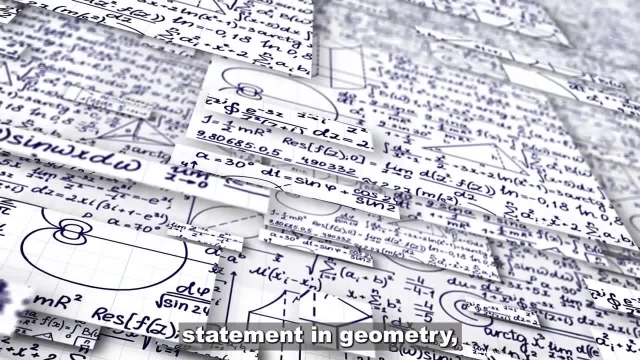 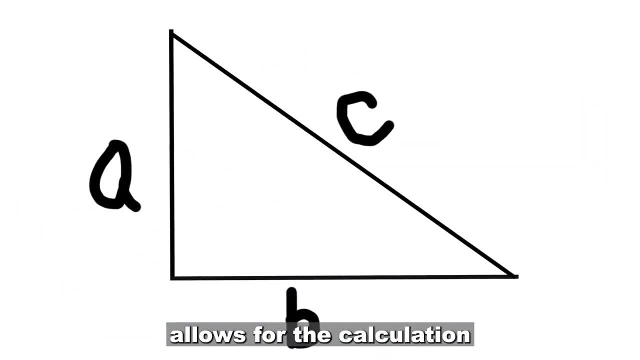 At first glance, the Pythagorean theorem may seem like a mere statement in geometry, but it actually has a lot of important real-life applications. For instance, the theorem allows for the calculation of the length of a diagonal that connects two straight lines. 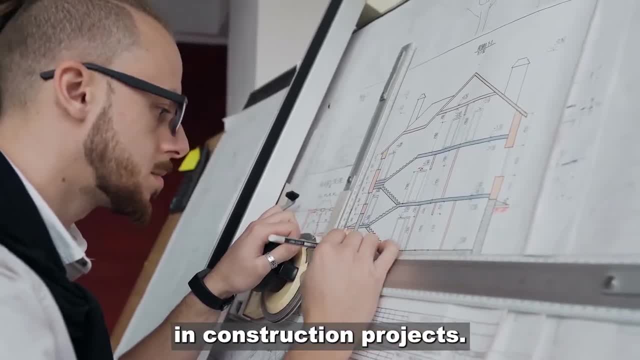 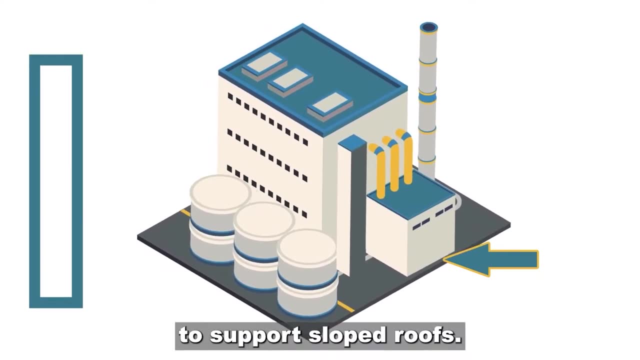 which is a formula often used by architects in construction projects. Not only does it help ensure that buildings are square, but it also determines the size of beams to support sloped buildings. Besides this, the Pythagorean theorem is also used in meteorology and. 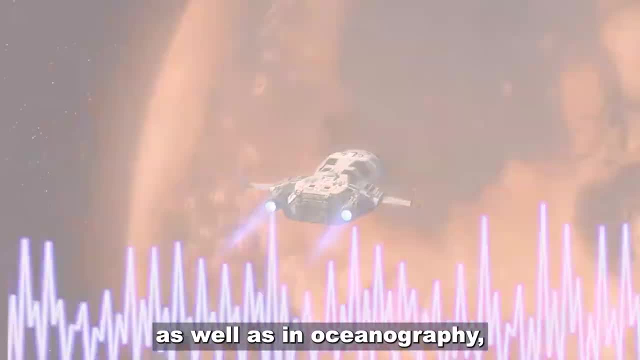 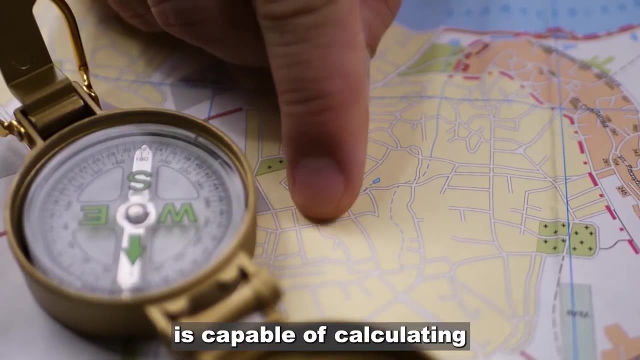 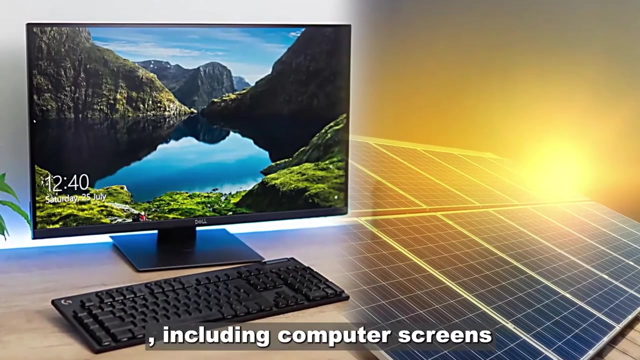 aerospace to determine the source of sound and its range, as well as in oceanography, to help scientists calculate the speed of sound waves in water. In navigation, it is capable of calculating the shortest distance between two given points and can also determine the dimension of electronic devices, including computer screens and solar panels. 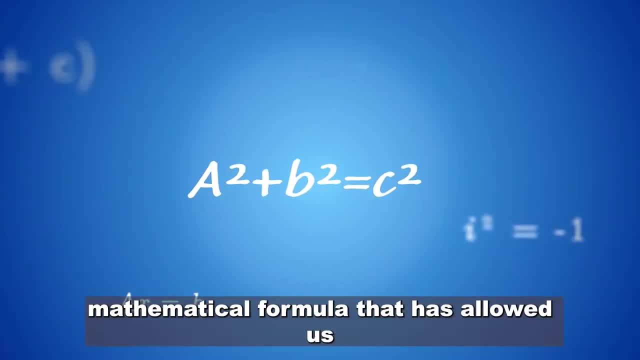 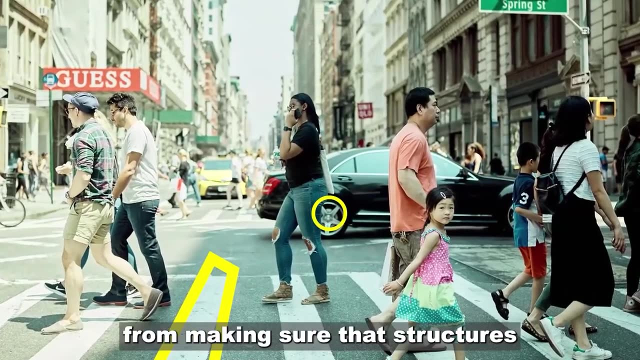 Without a doubt, the Pythagorean theorem is an incredible mathematical formula that has has allowed us to deepen our understanding of the world. More than that, though, it has helped us improve our everyday lives, from making sure that structures are safe and sound. 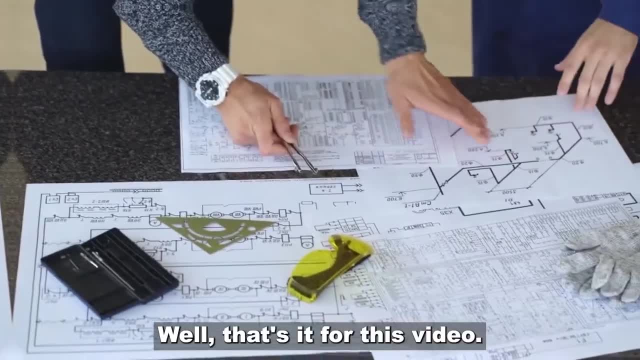 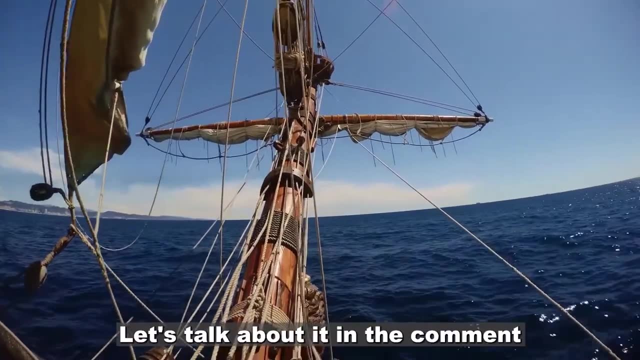 to helping us plot routes and chart direction. Well, that's it for this video. Have you had to use the Pythagorean Theorem for school, for work, or maybe both. Let's talk about it in the comments section down below. Don't.